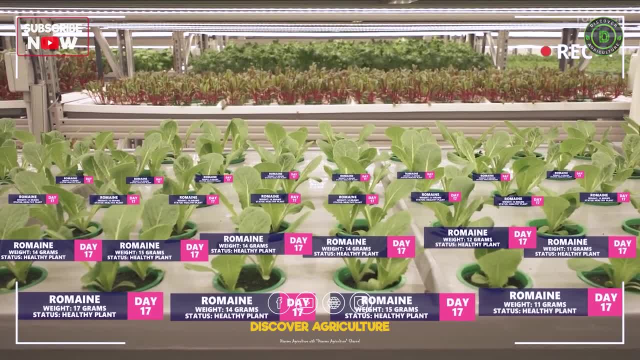 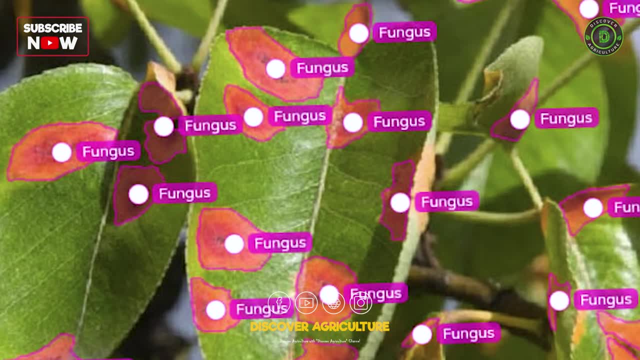 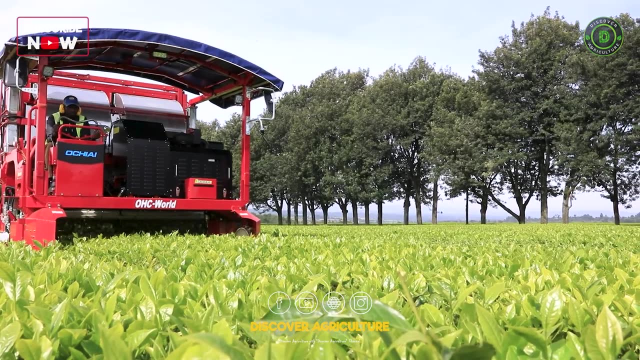 data on crop growth and help them identify any issues before they become major problems. By monitoring crop health, farmers can take proactive steps to prevent crop damage and ensure a healthy harvest. 2. Precision Farming. Precision farming involves the use of AI algorithms to analyze data. 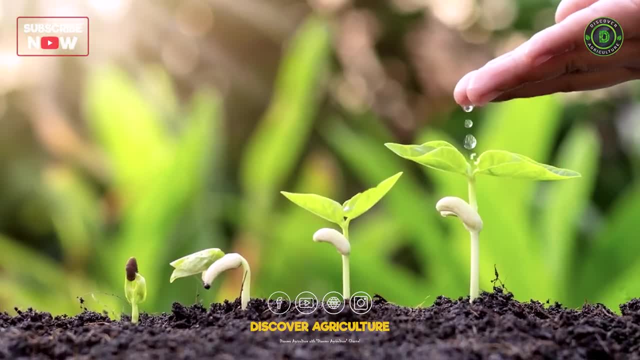 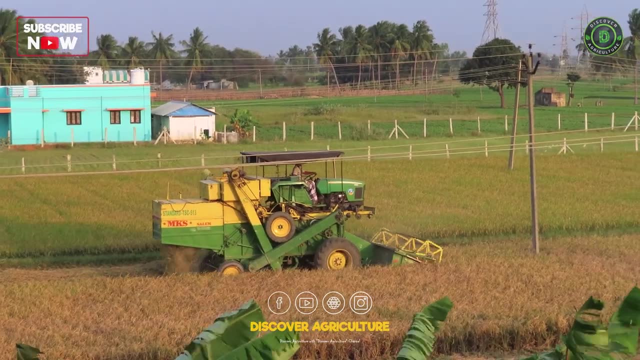 on what is happening in the crop. This technology can provide farmers with real-time data on crop growth, soil quality and weather patterns and crop growth to optimize planting, fertilizing and harvesting. This technology can help farmers optimize their crop yields and reduce waste by 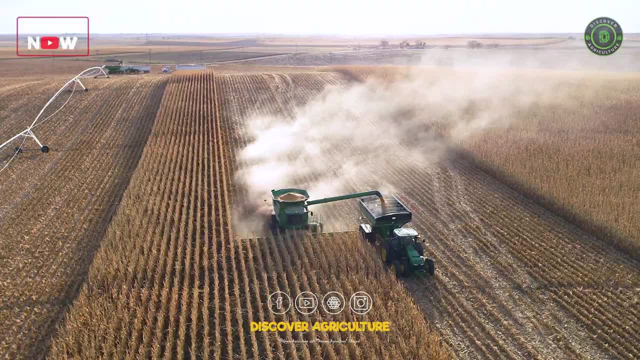 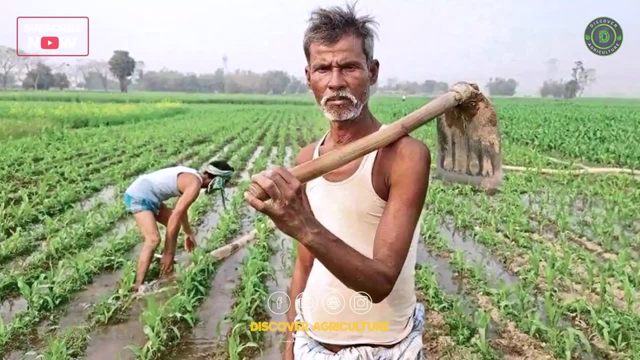 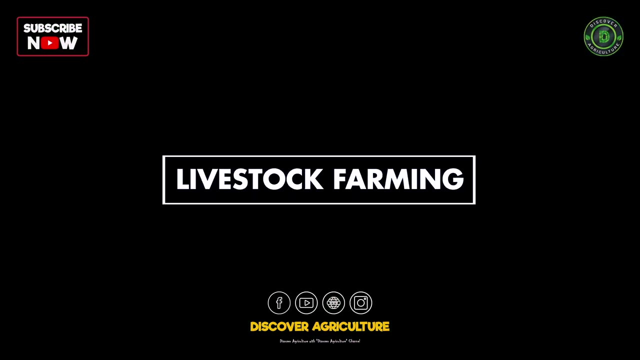 identifying the best time to plant, fertilize and harvest crops. By analyzing data on weather patterns and soil quality, farmers can also make informed decisions on the type and amount of fertilizers and pesticides to use. 3. Farming: 3. AI in Livestock Farming. Livestock monitoring involves the use of AI-powered 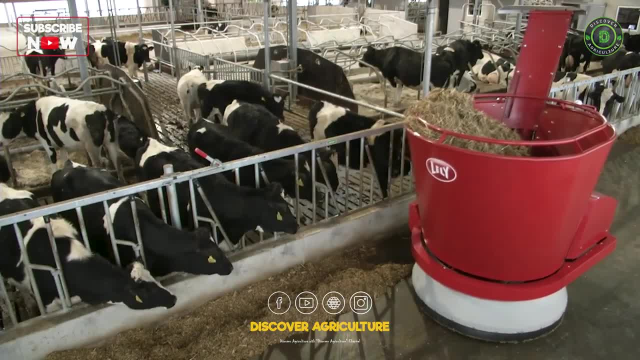 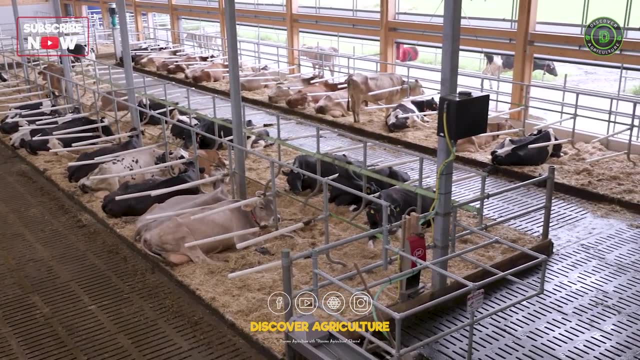 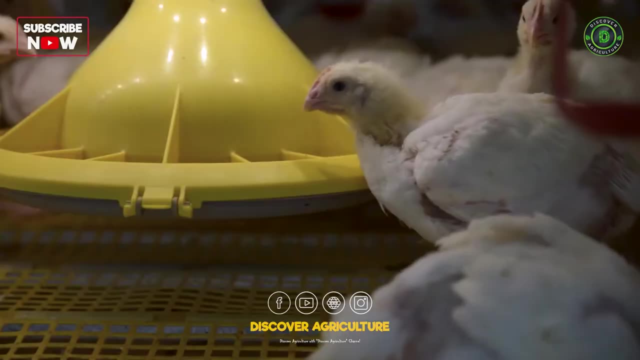 sensors to monitor the health behavior and feeding patterns of livestock. This technology can help farmers identify any health issues before they become major problems and optimize feed and water usage. By monitoring livestock behavior, farmers can also identify any issues with feeding or watering systems. 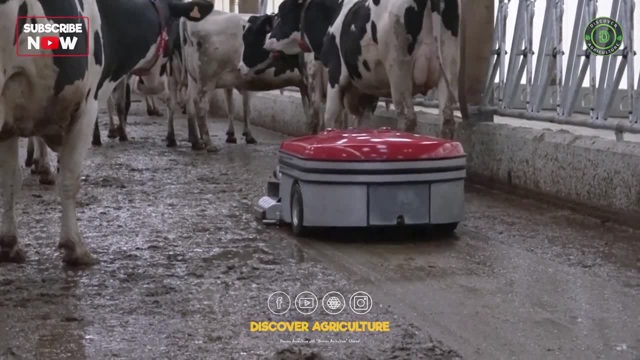 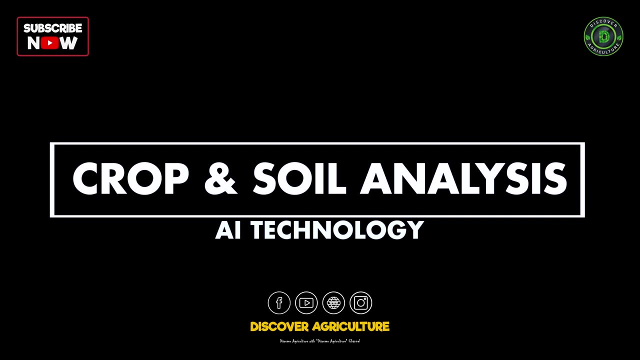 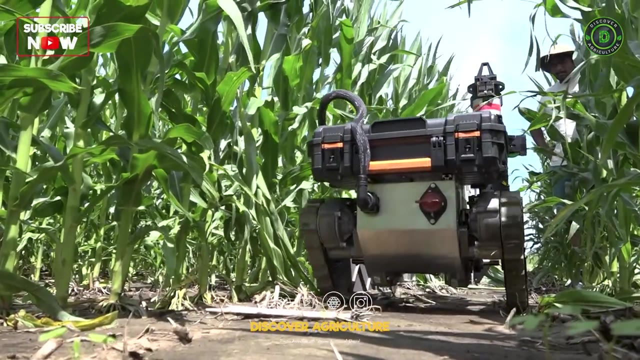 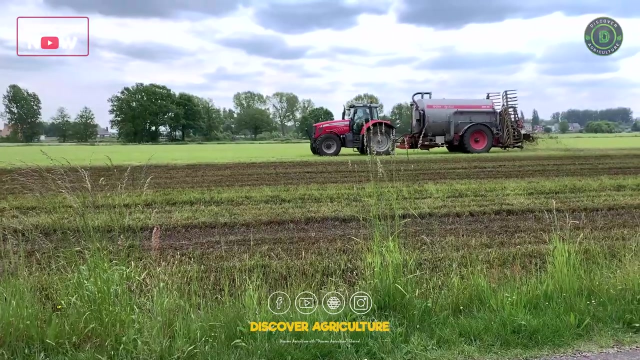 systems. AI technologies can be used to farm waste management, in feed management and to milk the animals. 4. Crop and Soil Analysis. Crop and soil analysis involves the use of AI algorithms to analyze data on soil samples to determine nutrient levels and recommend optimal fertilizer use. This technology can help farmers. 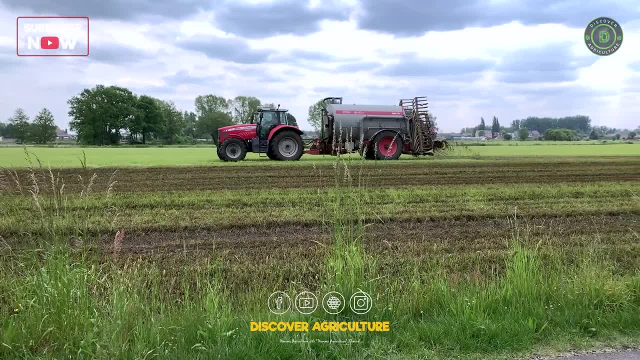 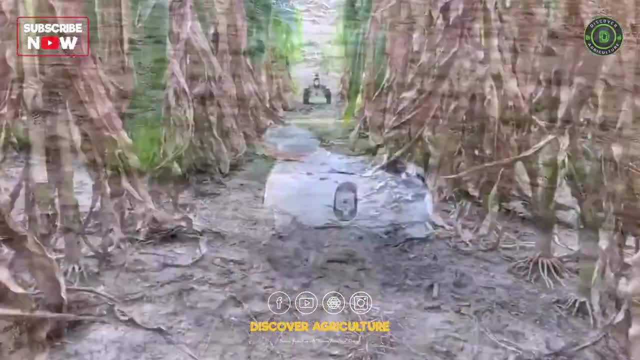 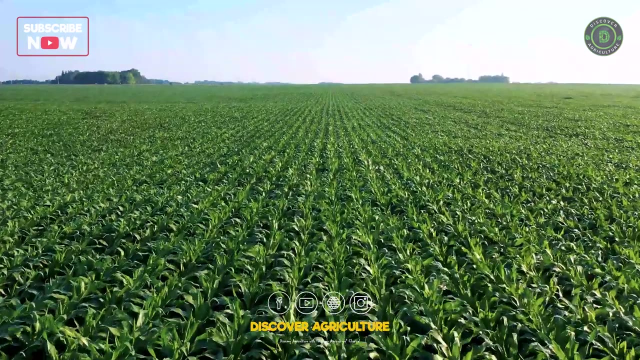 optimize their crop yields and reduce waste by identifying the best type and amount of fertilizers to use. By analyzing data on soil quality, farmers can also make informed decisions on which crops to plant and how to manage their fields. 5. Crop Forecasting. 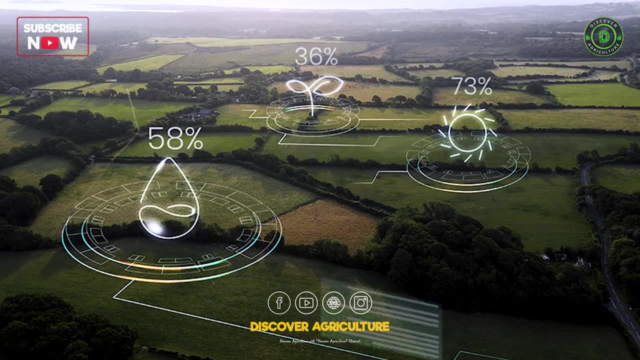 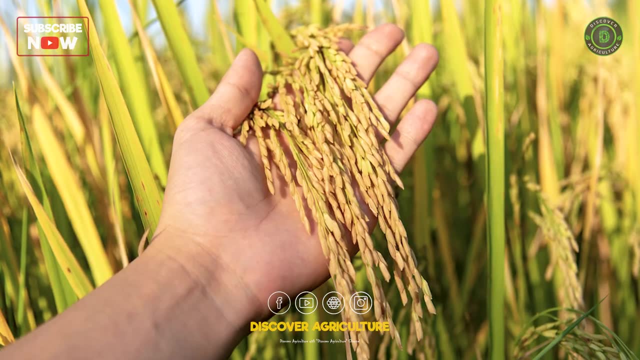 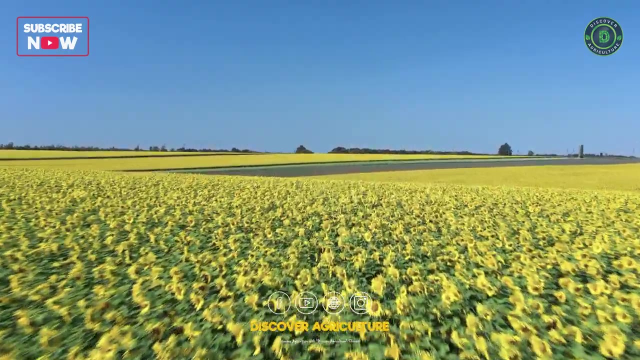 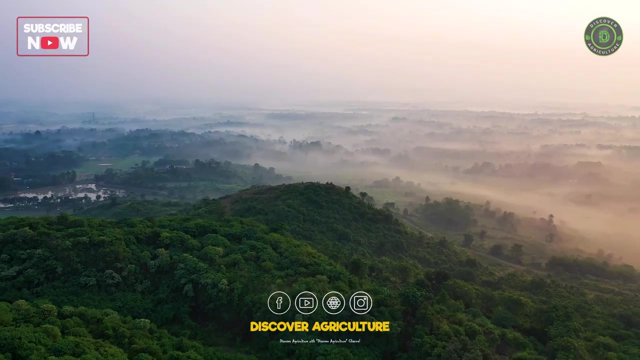 Crop forecasting involves the use of AI algorithms to analyze data on weather patterns, soil quality and crop growth to forecast crop yields. This technology can help farmers plan for the future and make informed decisions on when to plant and harvest crops. By forecasting crop yields, farmers can also make informed decisions. 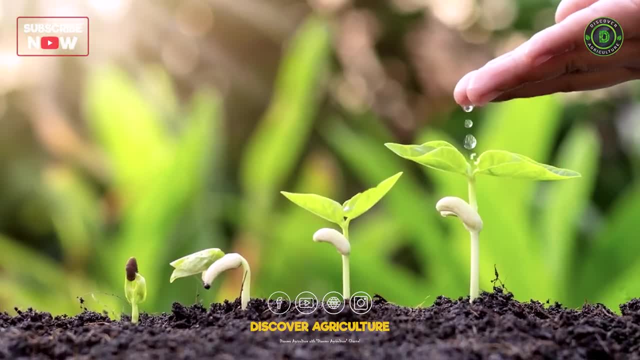 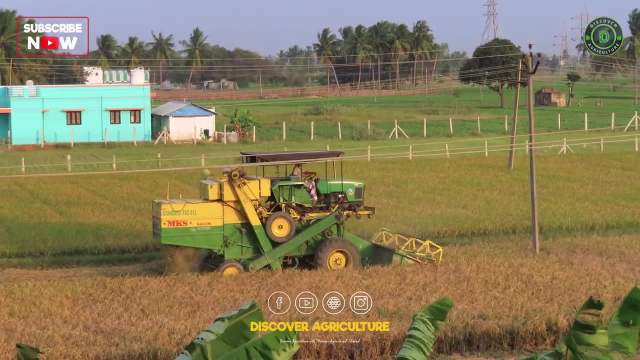 on what is happening in the crop. This technology can provide farmers with real-time data on crop growth, soil quality and weather patterns. soil quality and crop growth to optimize planting, fertilizing and harvesting. This technology can help farmers optimize their crop yields. 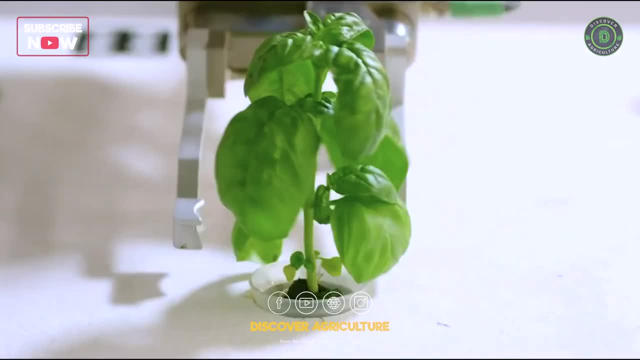 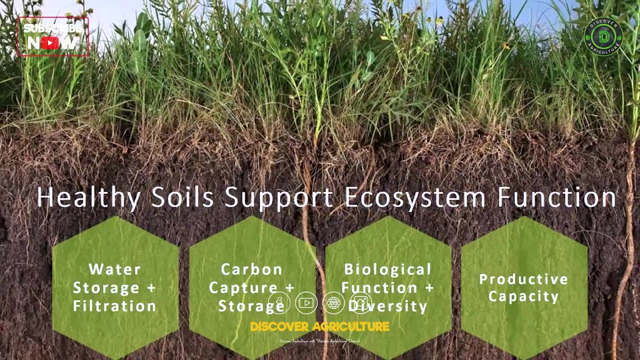 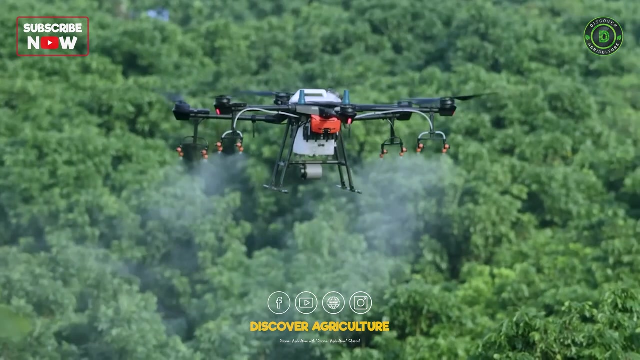 and reduce waste by identifying the best time to plant, fertilize and harvest crops. By analyzing data on weather patterns and soil quality, farmers can also make informed decisions on the type and amount of fertilizers and pesticides to use. 3. AI in Livestock Farming. 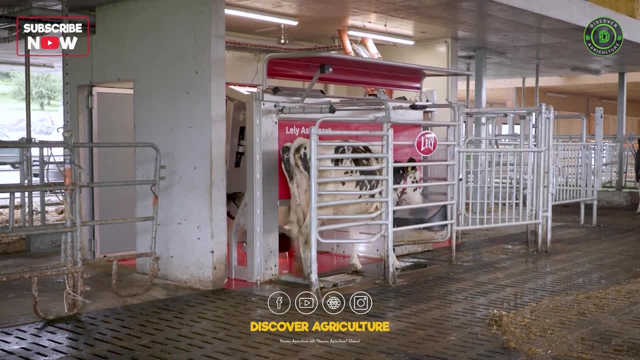 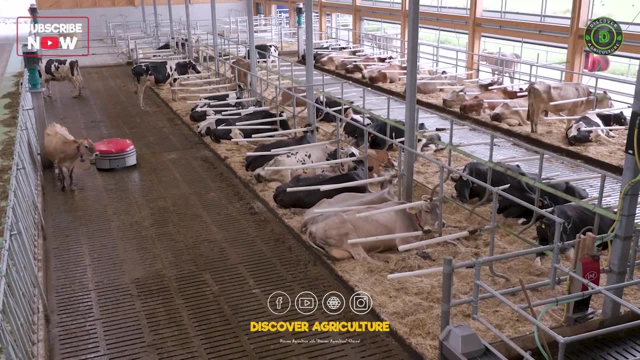 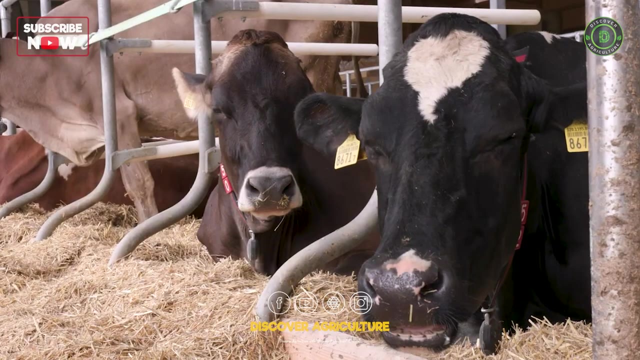 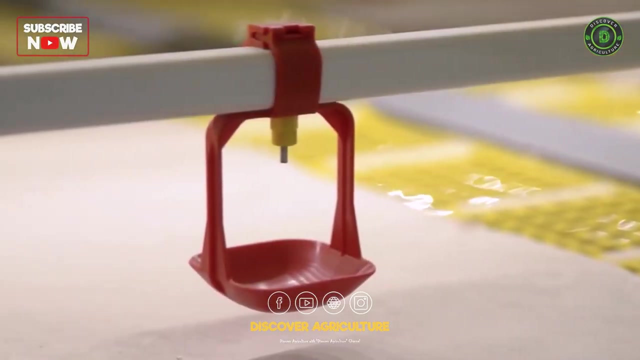 Livestock monitoring involves the use of AI-powered sensors to monitor the health, behavior and feeding patterns of livestock. This technology can help farmers identify any health issues before they become major problems and optimize feed and water usage. By monitoring livestock behavior, farmers can also identify any issues with feeding or watering. 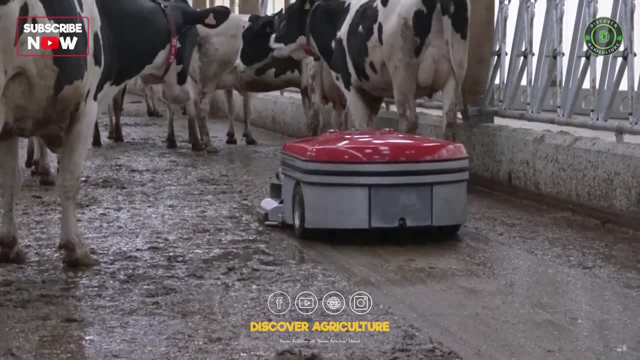 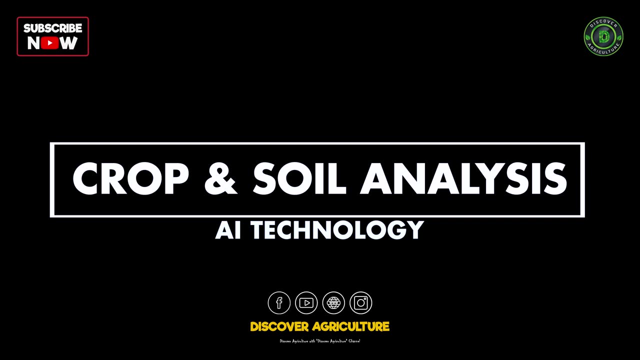 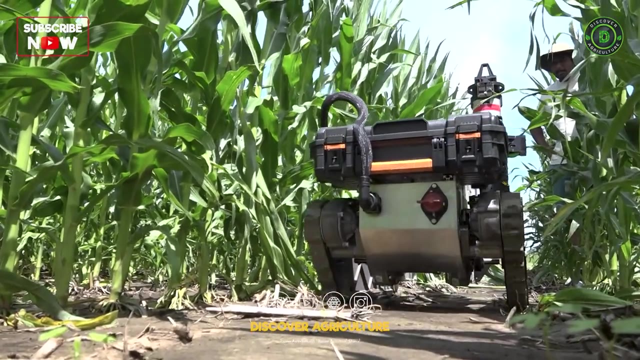 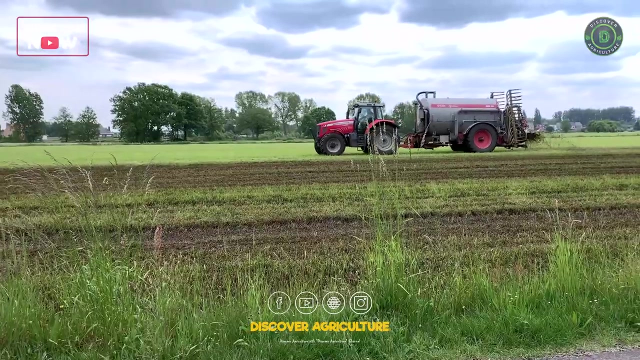 systems. AI technologies are can be used to farm waste management, in feed management and to milk the animals. 4. Crop and Soil Analysis. Crop and soil analysis involves the use of AI algorithms to analyze data on soil samples to determine nutrient levels and recommend optimal fertilizer use. This technology can help farmers. 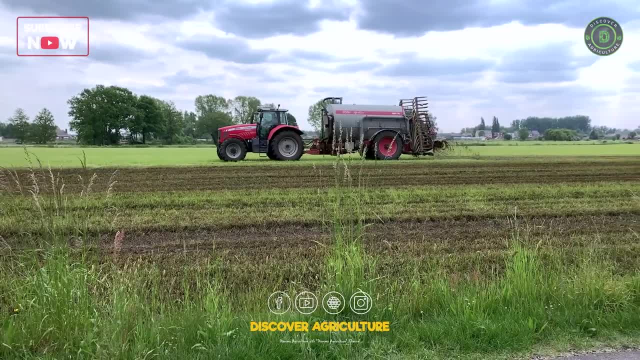 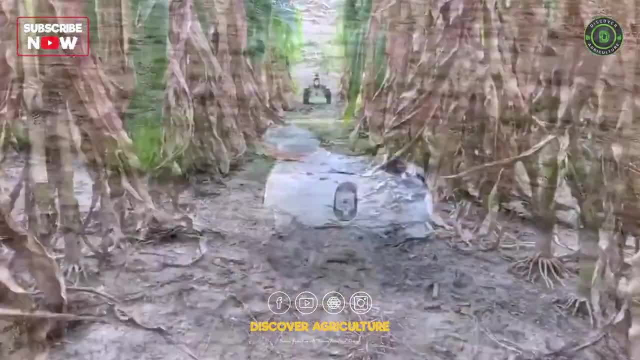 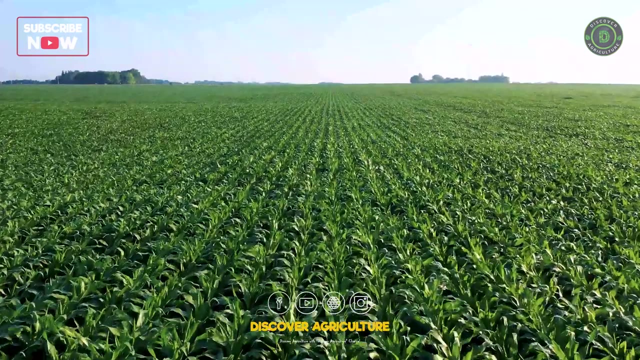 optimize their crop yields and reduce waste by identifying the best type and amount of fertilizers to use. By analyzing data on soil quality, farmers can also make informed decisions on which crops to plant and how to manage their fields. 5. Crop Forecasting. 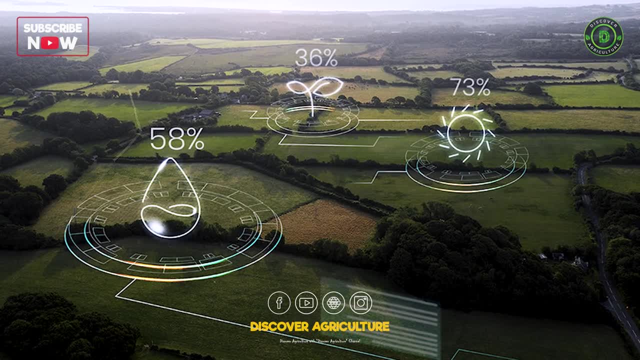 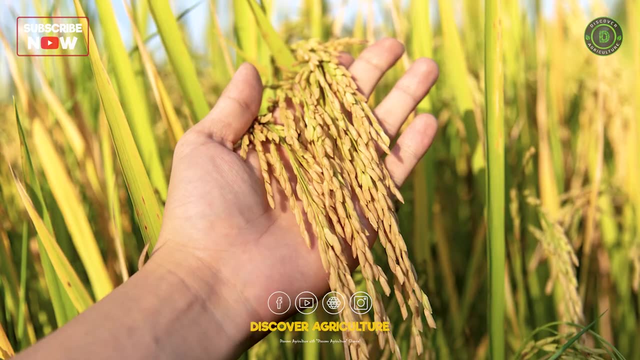 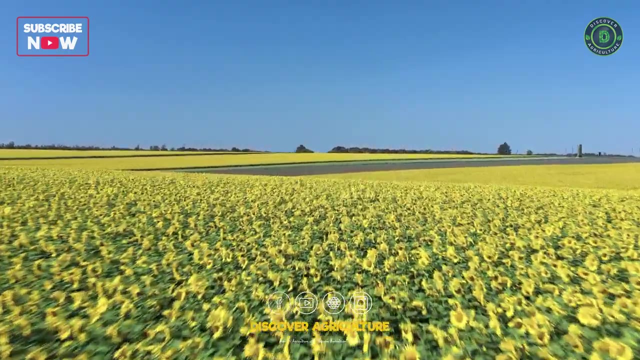 Crop forecasting involves the use of AI algorithms to analyze data on weather patterns, soil quality and crop growth to forecast crop yields. This technology can help farmers plan for the future and and make informed decisions on when to plant and harvest crops By forecasting crop yields. 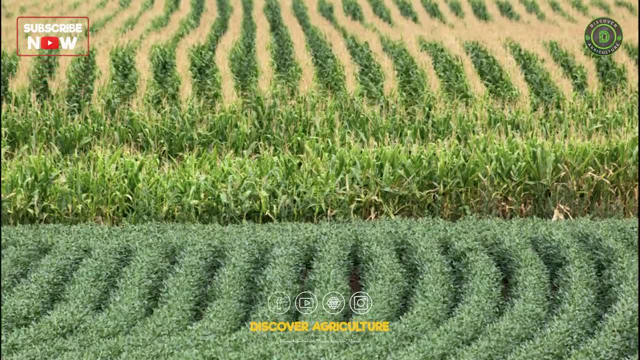 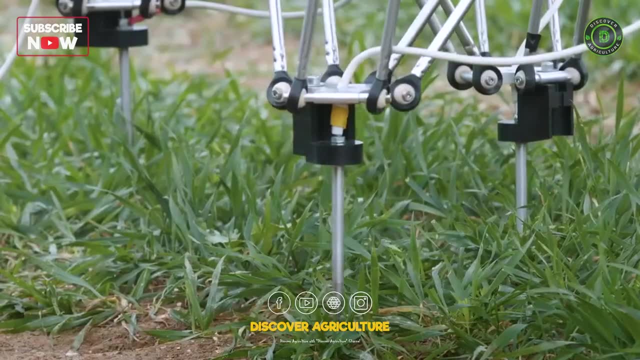 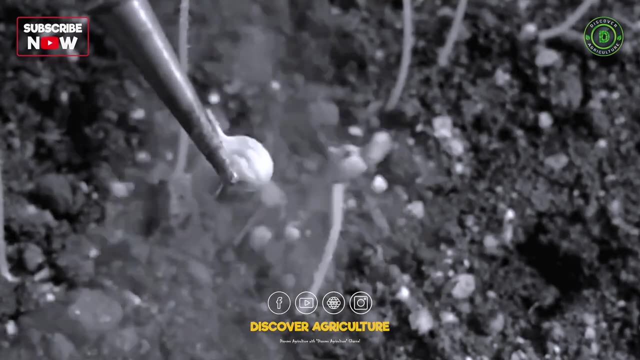 farmers can also make informed decisions on which crops to plant and how to manage their fields. 6. Weed and Pest Detection. Weed and pest detection involves the use of AI-powered cameras and sensors to detect and identify weeds and pests in crops. This technology can help. 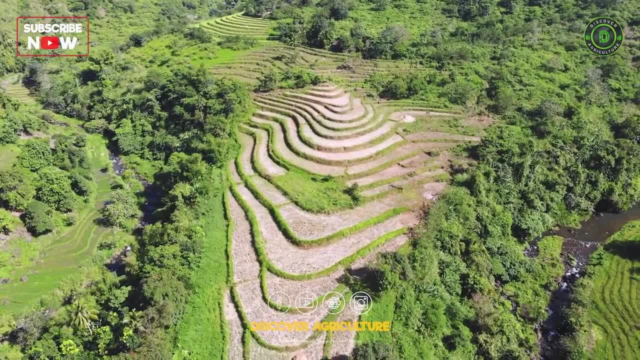 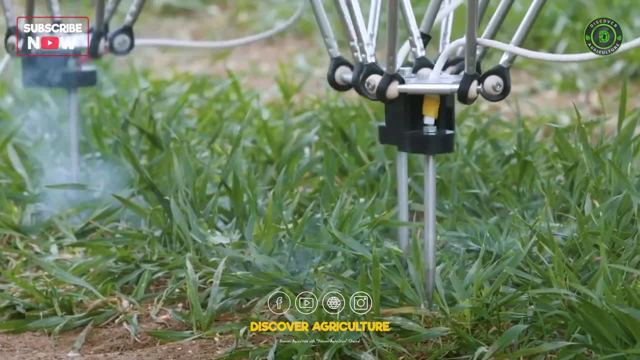 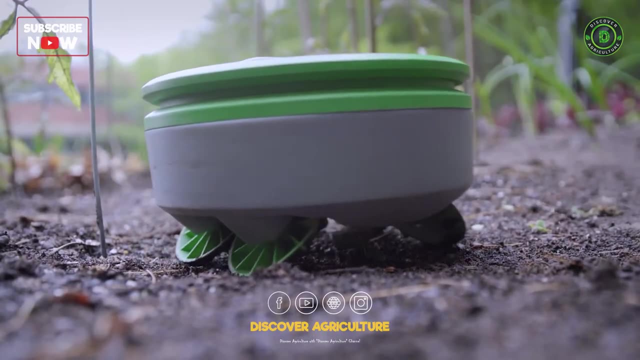 on which crops to plant and how to manage their fields. 6. Weed and Pest Detection. Weed and pest detection involves the use of AI-powered cameras and sensors to detect and identify weeds and pests in crops. This technology can help farmers take corrective action before the damage is done and reduce the 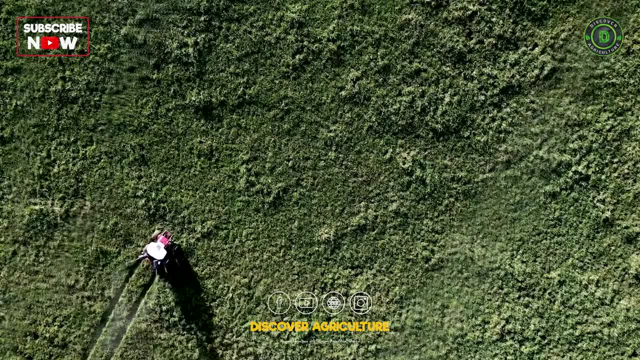 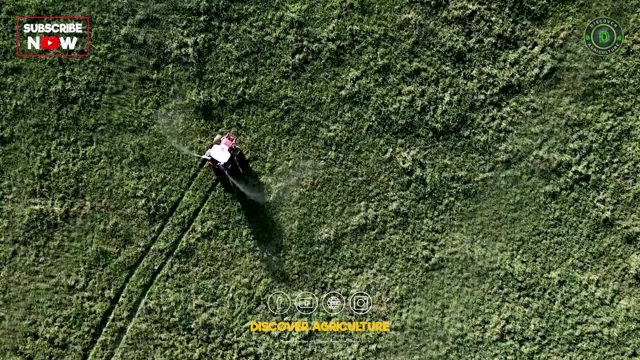 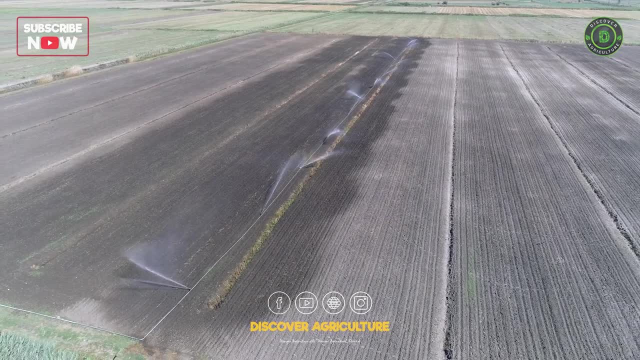 amount of pesticides used. By detecting and identifying weeds and pests, farmers can also make informed decisions on which crops to plant and how to manage their fields. 7. Irrigation Management. Irrigation management involves the use of AI algorithms to analyze data on weather patterns. 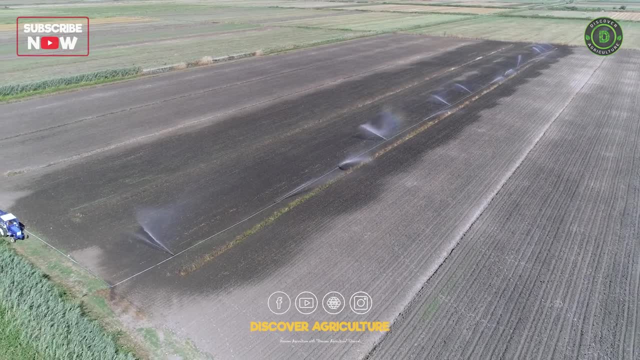 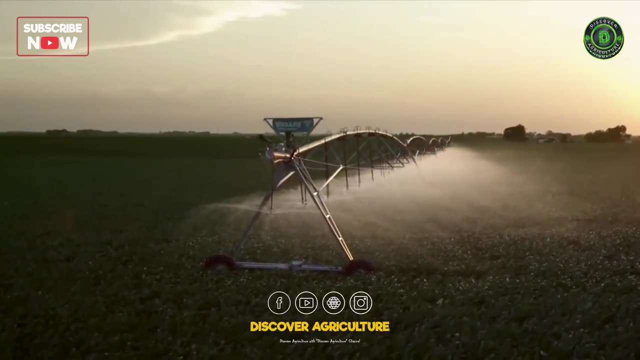 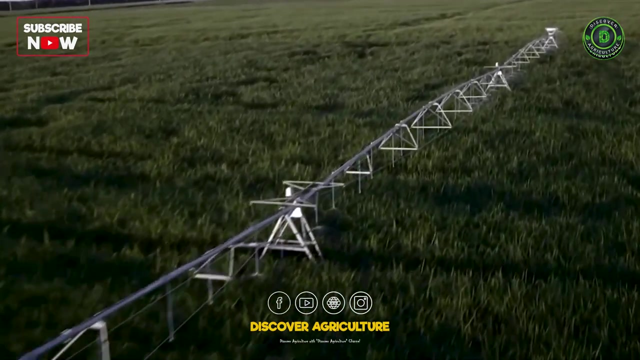 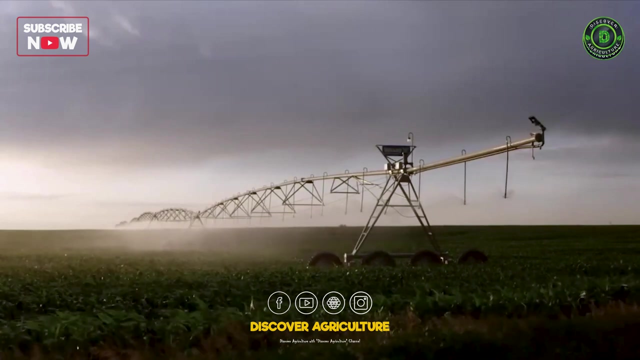 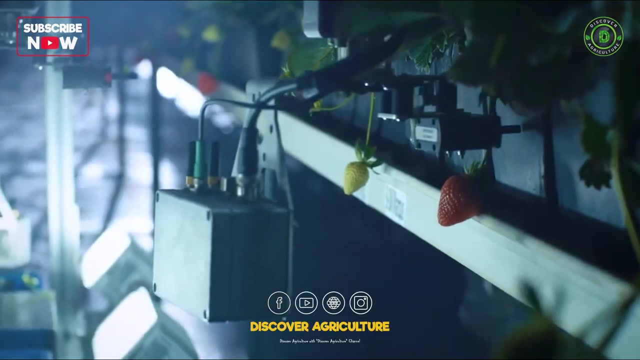 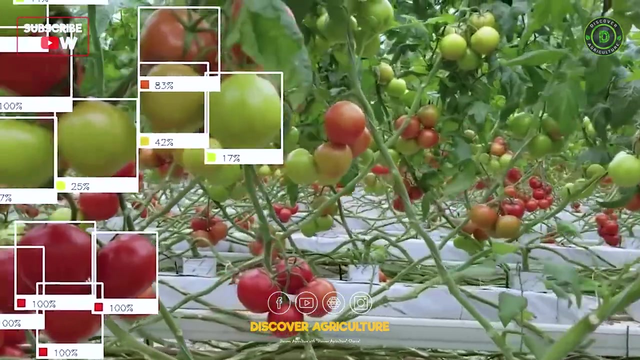 soil quality and crop growth to predict crop yields. This technology can help farmers take concrete steps to increase or ruined crop yields By Как interest把 robots to harvest crops, reducing the need for manual labor and increasing efficiency. This technology can help farmers save time and money by reducing the need for manual 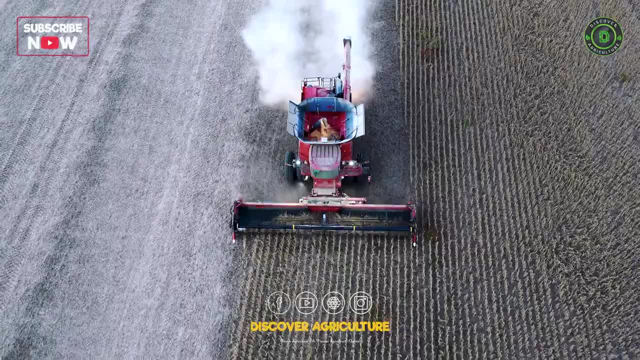 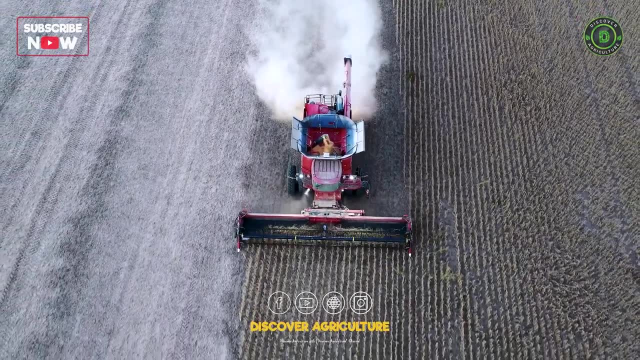 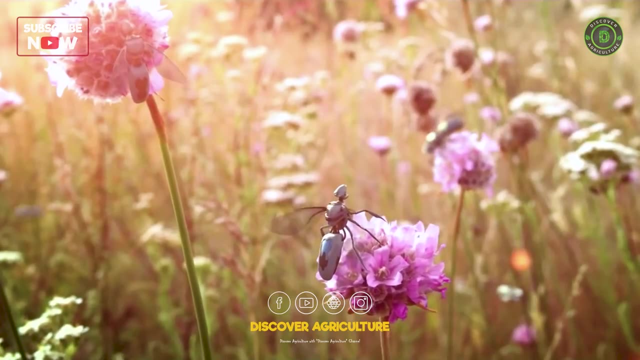 labor and improving the quality of the harvest. By using AI-powered robots, farmers can also reduce the risk of injury to workers and improve safety in the field. 9. Pollination: Pollination involves the use of AI-powered drones that can mimic the pollination behavior of bees. 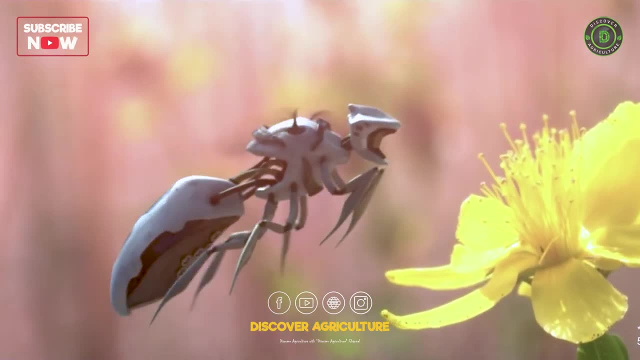 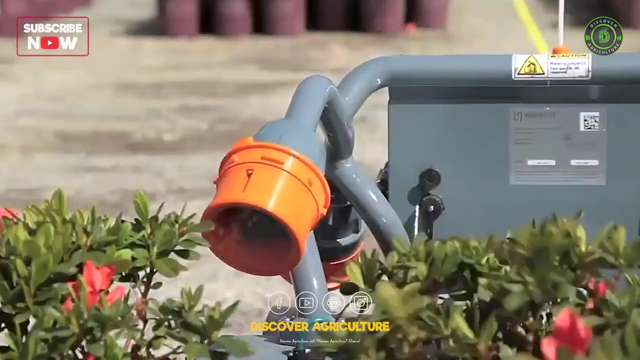 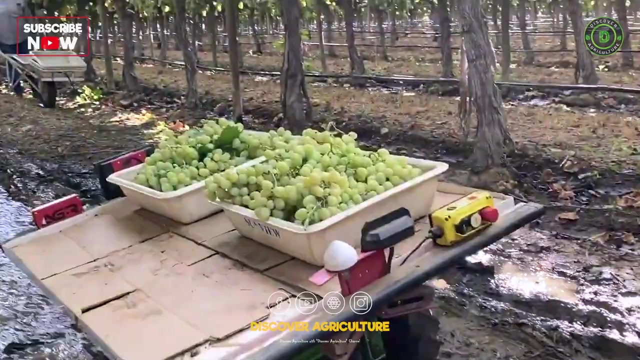 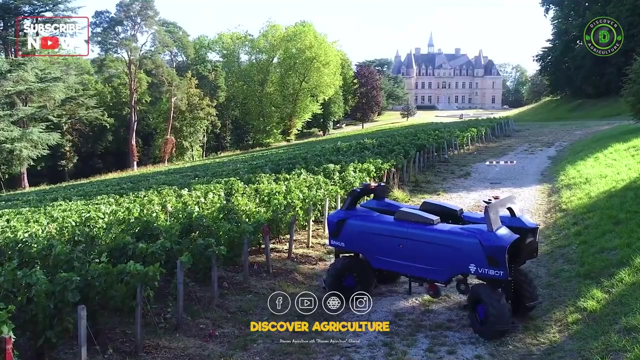 These drones are equipped with cameras and sensors that can detect flowers. In conclusion, these technologies have the potential to increase productivity, reduce costs and optimize crop production. AI technology is transforming the agricultural industry and holds great potential for the future of sustainable and efficient agriculture. 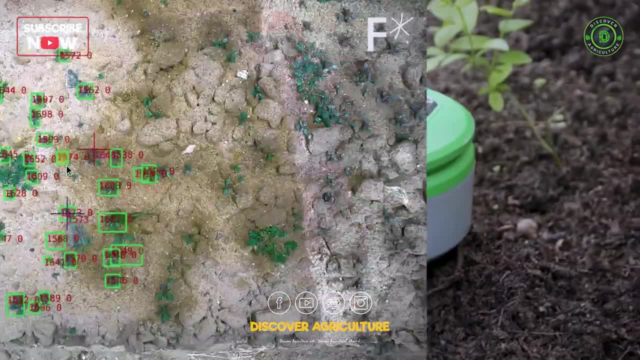 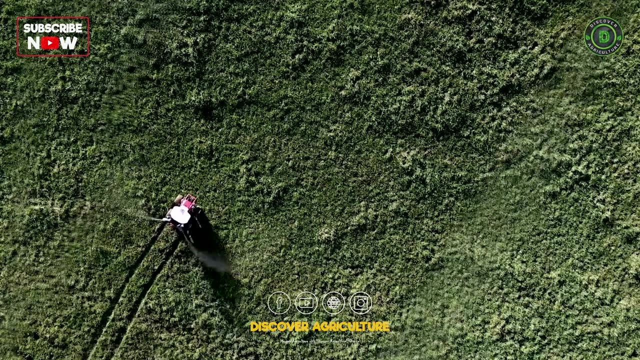 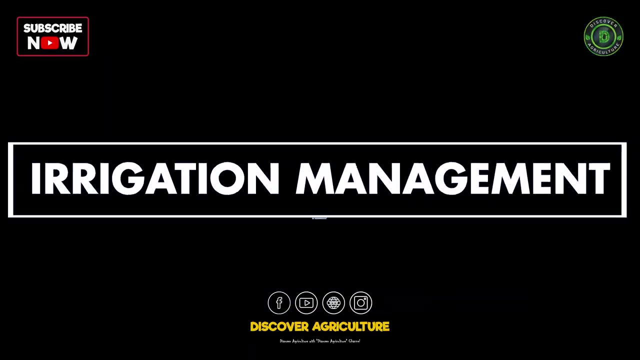 farmers take corrective action before the damage is done and reduce the amount of pesticides used. By detecting and identifying weeds and pests, farmers can also make informed decisions on which crops to plant and how to manage their fields. 7. Irrigation Management- Irrigation. 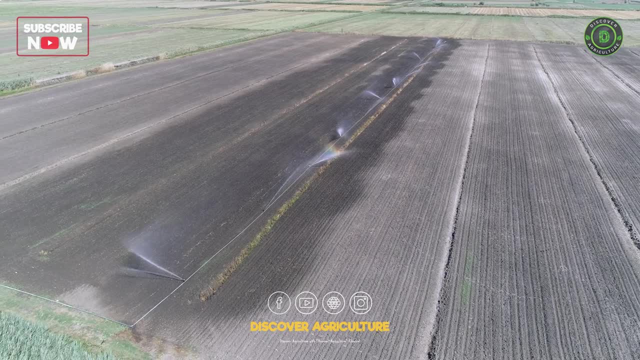 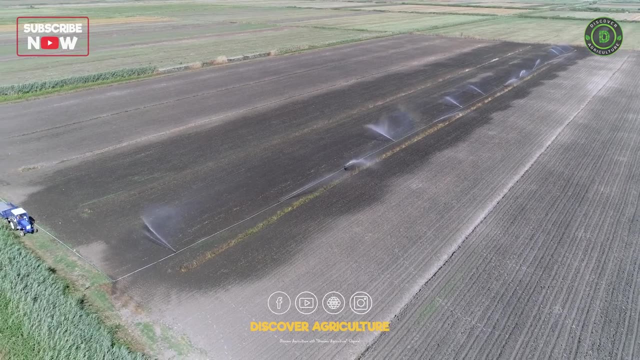 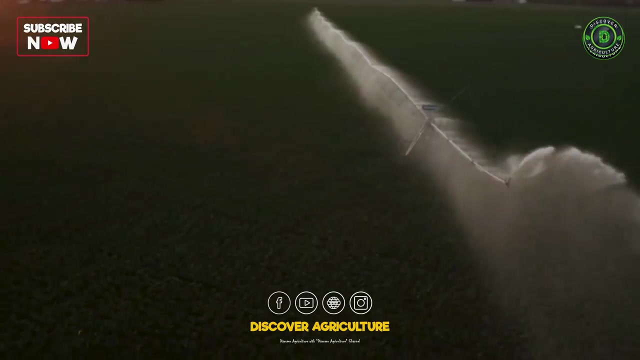 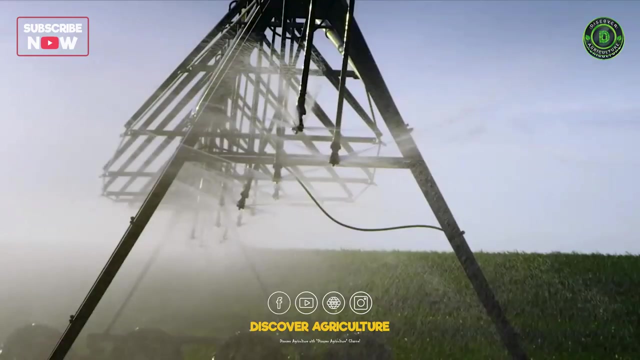 management involves the use of AI algorithms to analyze data on weather patterns, soil quality and crop growth to optimize irrigation systems. This technology can help farmers optimize their water usage and reduce costs by identifying the best time to irrigate crops By analyzing data on weather patterns and soil quality. 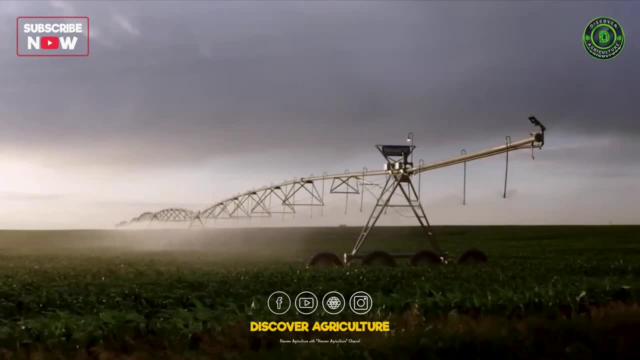 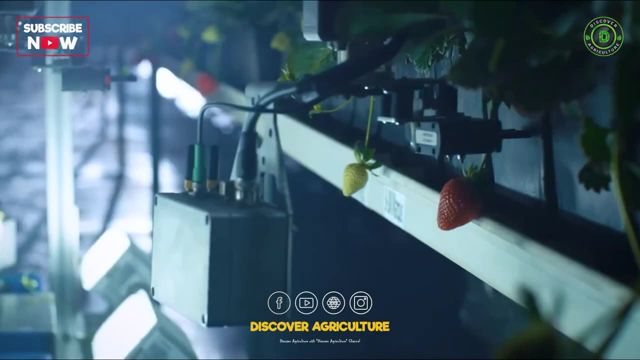 farmers can also make informed decisions on when to irrigate and how much water to use. 8. Harvesting: Harvesting involves the use of AI-powered robots to harvest crops, reduce the amount of water to be used and reduce the amount of water to be used. 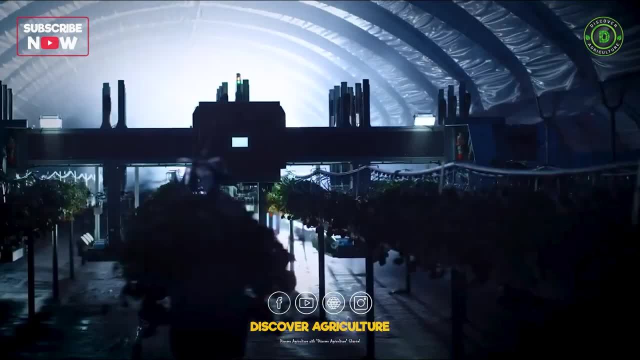 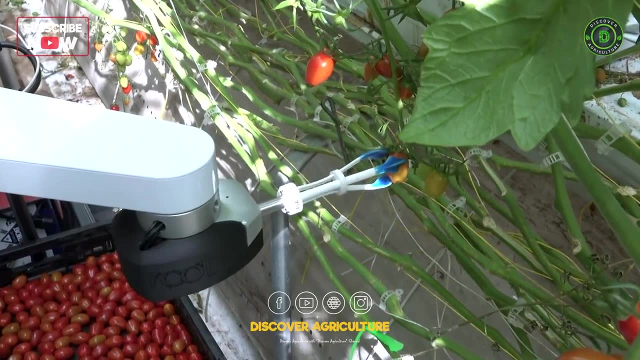 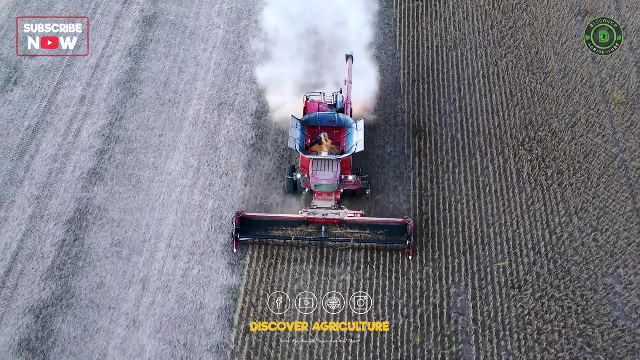 This technology can help farmers save time and money by reducing the need for manual labor and increasing efficiency. This technology can help farmers save time and money by reducing the need for manual labor and improving the quality of the harvest. By using AI-powered robots, farmers can also reduce the risk of injury to workers and improve safety in the field. 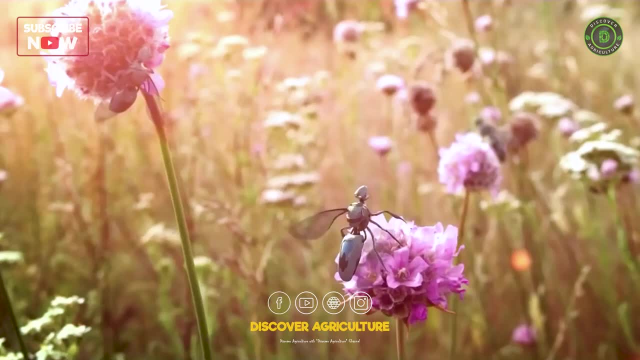 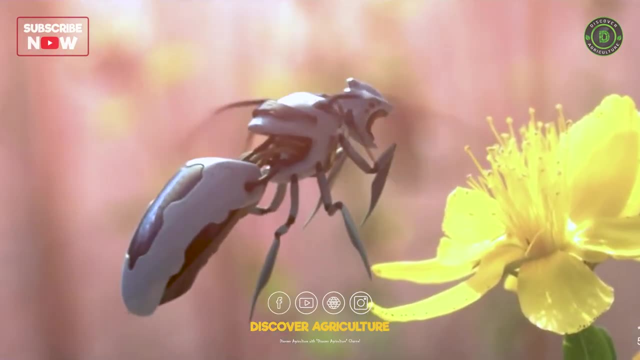 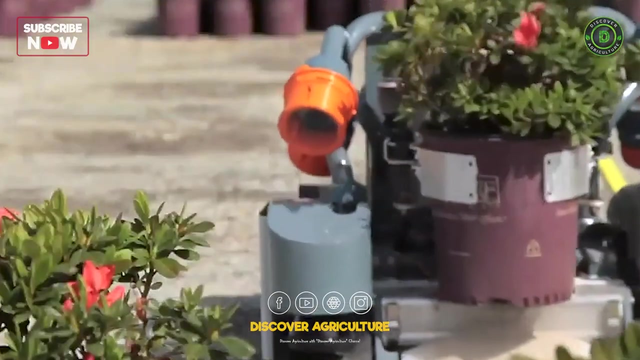 9. Pollination. Pollination involves the use of AI-powered drones that can mimic the pollination behavior of bees. These drones are equipped with cameras and sensors that can detect flowers. In conclusion, these technologies have the potential to increase productivity, reduce costs and optimize crop production. 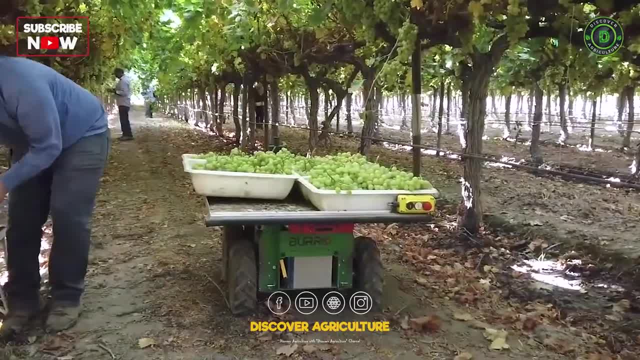 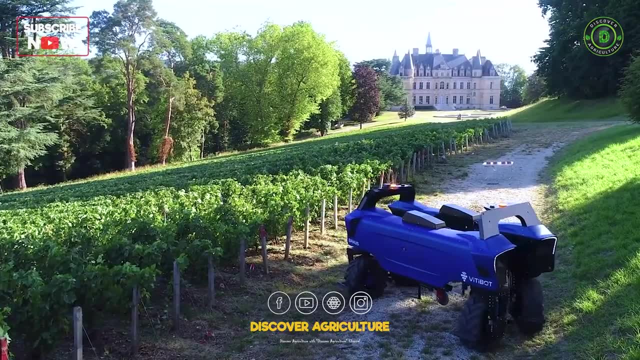 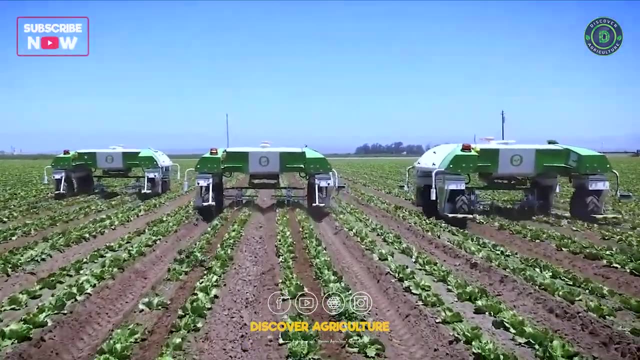 AI technology is transforming the agricultural industry and holds great potential for the future of sustainable and efficient agriculture. That's all for today's video on Artificial Intelligence in Agriculture. We hope you found it interesting and learned something new. If you enjoyed this video, please give it a thumbs up and share it with your friends. 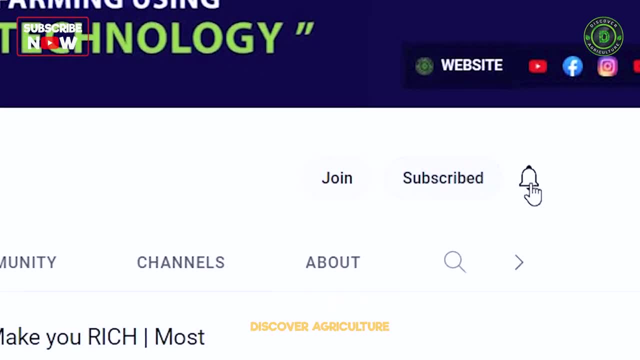 Don't forget to subscribe to our channel for more informative videos on agriculture and technology. Thank you for watching and have a great day.